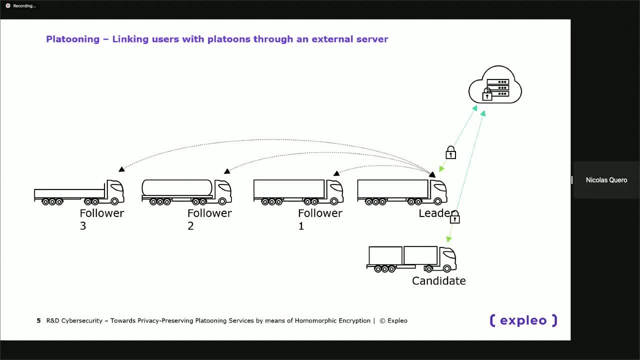 in a connection with a platoon nearby so that the user can follow this platoon and reach him somewhere. The problem is that the server needs to have access to the client's sensitive location data, and our idea was to use homomorphic encryption to privately connect the user with the platoon. 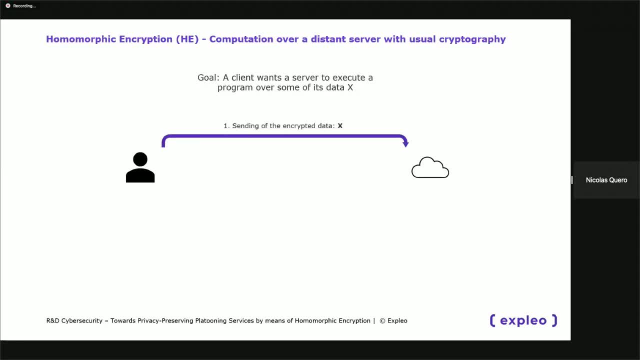 So, to tell you about homomorphic encryption, I recall to you how cryptography works. the usual cryptography works nowadays. So if a user wants to send some data to a server and the server wants to perform some operations over the client's data, what the user can do right now. 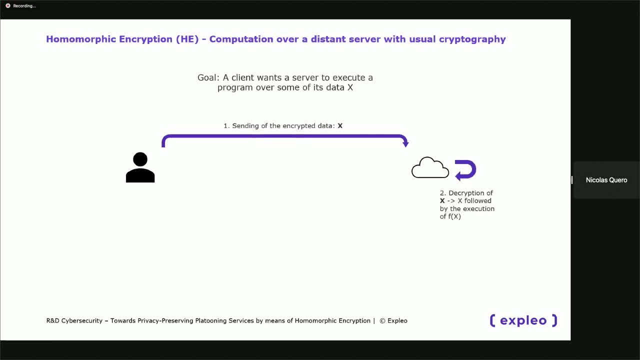 it can send encrypted data, but the server has to decrypt the data in order to perform some operations over the data from the user, and then it gets sent back the results in an encrypted form. but the problem is that the server needs to access this data and the homomorphic encryption. 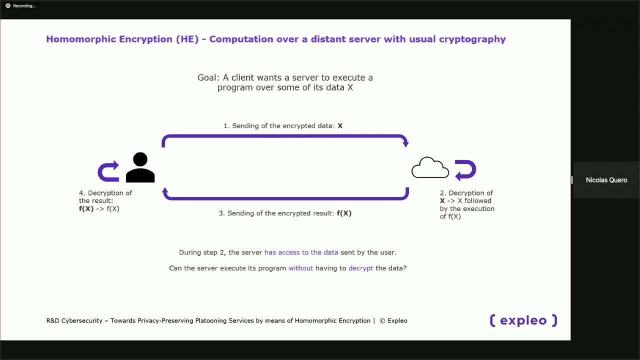 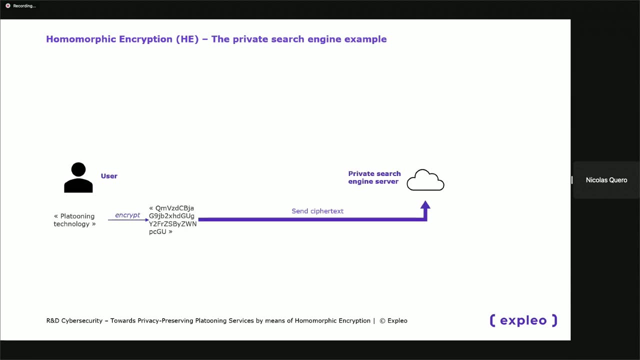 aims at preventing this decryption state on one server side and to only use encrypted data at all points. So the first example would be a search engine over a server where the user could send the nick from the encryption of its query and the server, in order to send it back to the client, could drive spacecrafts to clouds. 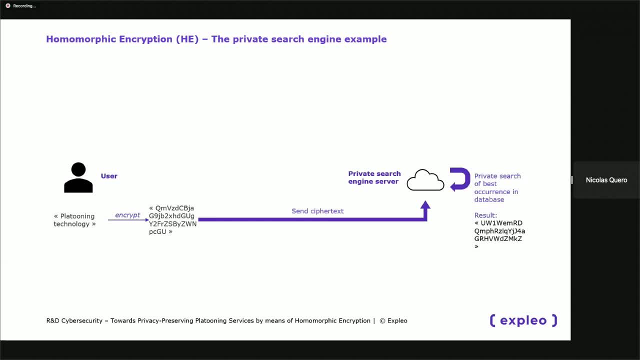 encryption of its query and the server could give a result to the client without accessing the data inside the query. So it would only use the encrypted data and still be able to send back an encrypted result. This way, the server doesn't have to read what the user was asking for and the user would 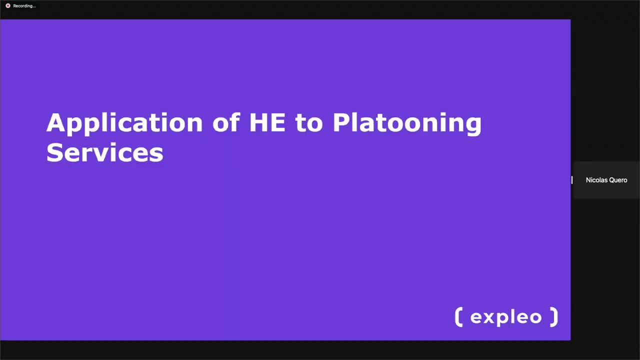 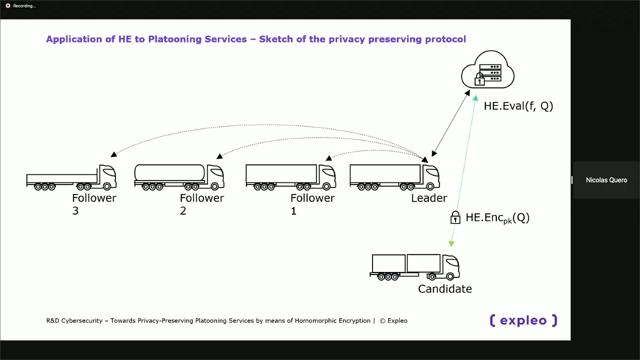 still be able to put to obtain its answer. So we wanted to use homomorphic encryption in order to create a plating service while maintaining privacy from the users data. So what we really do is we encrypt the data from the client homomorphic in our protocol, but after the server shares success to the 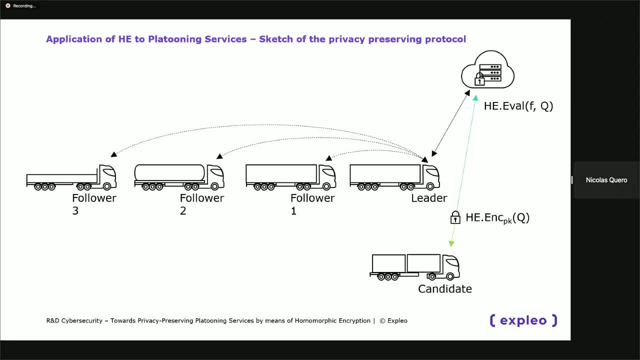 plate bones data, for example, you should the client, homomorphic in our protocol but in the server here, has access to the plate ones data. for example, you should data from the client, homomorphic in our protocol but in the server, share has. server would be having some platoons which would be which would agree to share some data with the 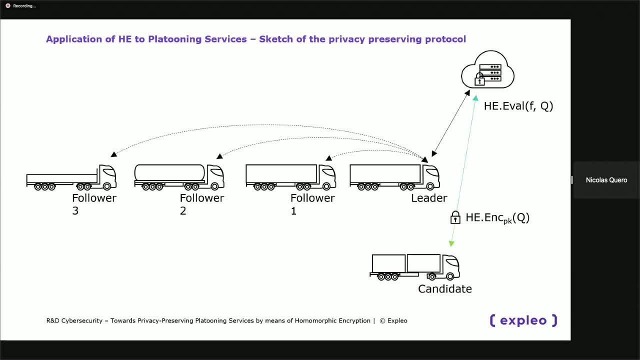 server, namely their positional data, but the users they would like to to stay private and not to share any data with the server. so the we assume that after that the server returns the, the platoon number that the user would have to reach, the user is able to privately know how to contact. 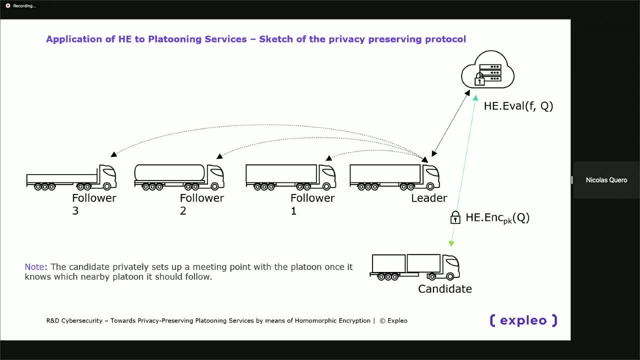 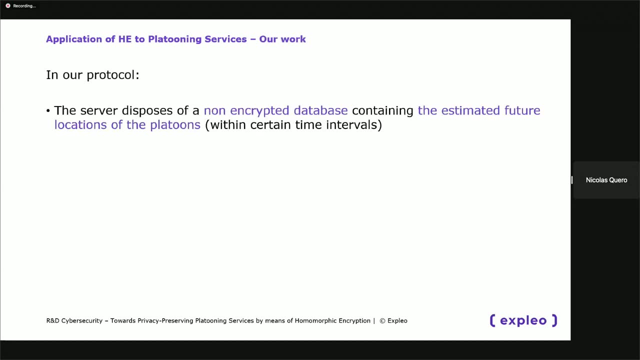 the platoon, for example with low range communication or some privacy preserving mechanism, that that can be up to the choice of the implementation. so, as i said, the server disposes of a non-encrypted database with the platoon informations and, instead of disclosing the the position of the position of the client to the server directly. 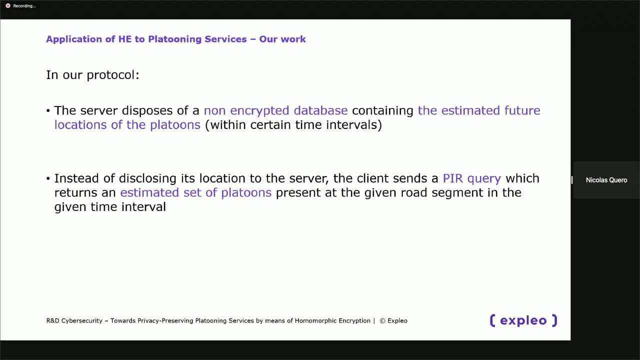 what we do is we make the client perform a PRO query to to the server, and the PRO query principle, which i will describe to you just after. that, means that someone with a PRO query can obtain a precise element of the database without disclosing to the server which element it wants to to obtain and instead of disclosing the precise position from the client. 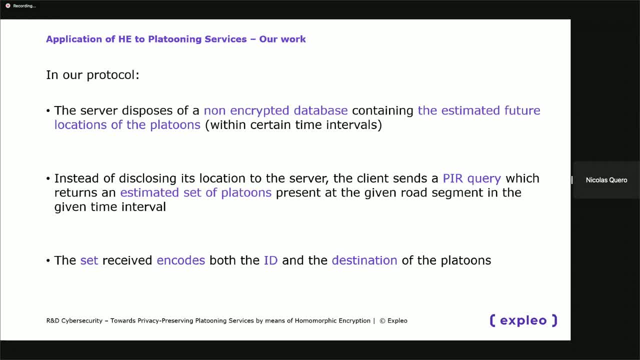 in this destination. what we do is we estimate the future locations of the platoons. for example, the the button has a fixed or any user on the road normally knows that in 10 minutes it should be in, like the road a5, segment 10. let's say so. 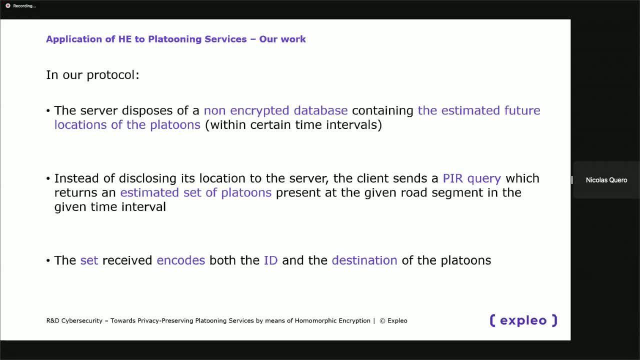 we give to the server, the platoons give to the server an estimation of its future location and what the client does? it performs a PRO query over this estimation. say, the user will ask to to the server, who will be in the same segment as him in 10 minutes. 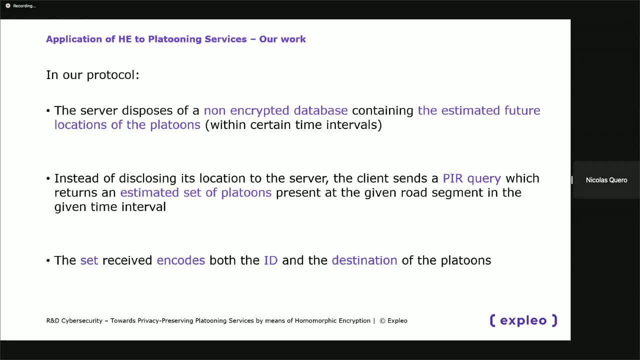 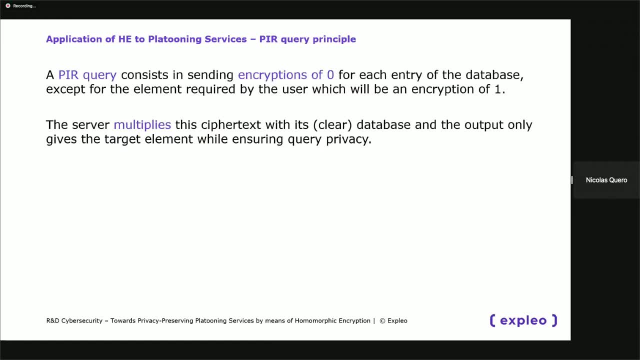 and the server with the PRO query will return to him this precise set of platoons privately. so to perform a PRO query, what we do is we send encryptions of zeros everywhere. so, for example, in the array which you have encrypt, you have zeros non-encrypted here, but they will be encrypted. 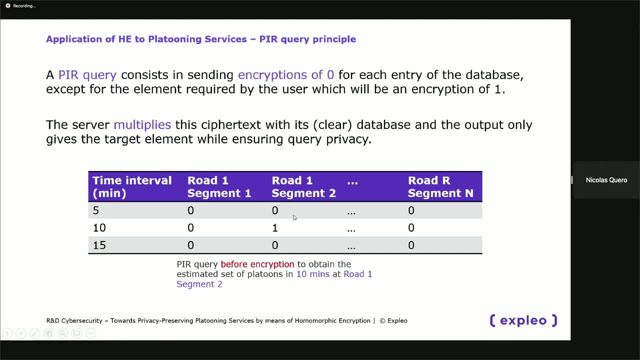 who work with each, except for one precise element, which will be a one. and then, when you perform a multiplication between this ciphertext and the database from the server, the output will be encryptions of zeros everywhere, so, for example, on the server here, everywhere, because zero times anything is zero. um, and one element, which will be 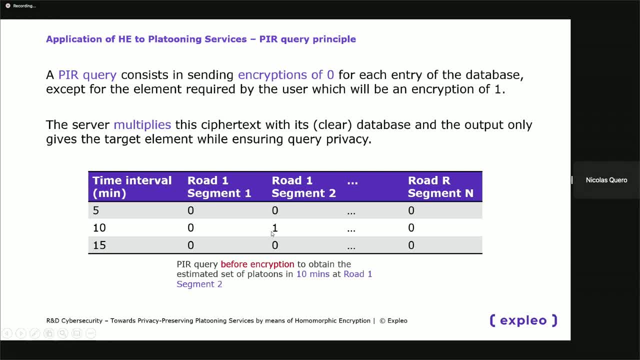 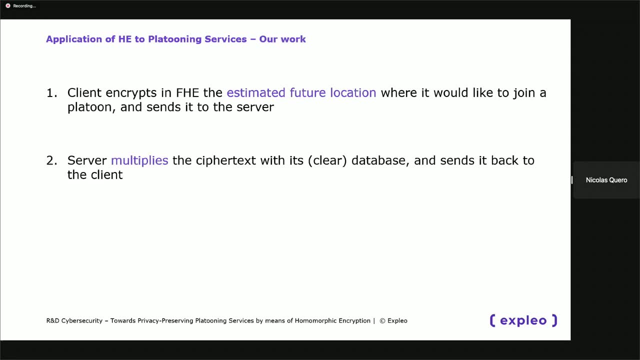 non-null, which is the element which is set to one from the client. of course, the this array is encrypted, so the server cannot see which element is one and which one is zero. so, as i said, the gland first encrypts its uh, the, the estimate future. estimated future location. 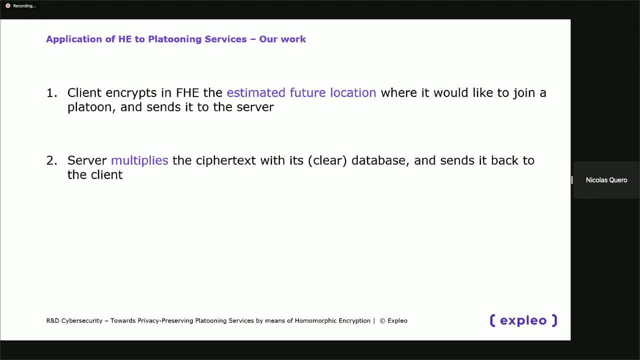 where it would like to meet a platoon and send it to the server. the server performs the pro query by multiplying the ciphertext with its database and then it sends the result back to the client. then this: the client obtains a set of platoons which encodes both the id from the platform. 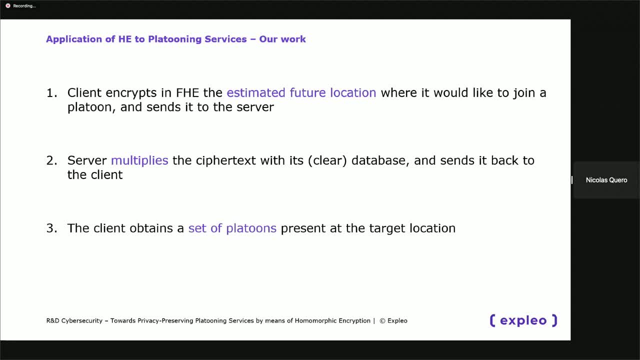 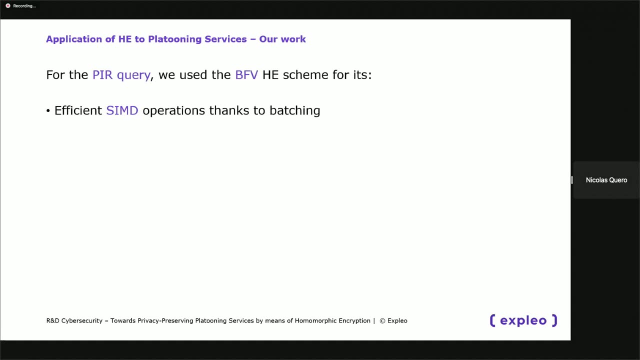 and its destination and with this set the client is able to know whether there is a platoon that's interesting him at the target location. so for the prior query we just did a homomorphic encryption scheme. we could use any additively homomorphic encryptions homomorphic encryption scheme to do 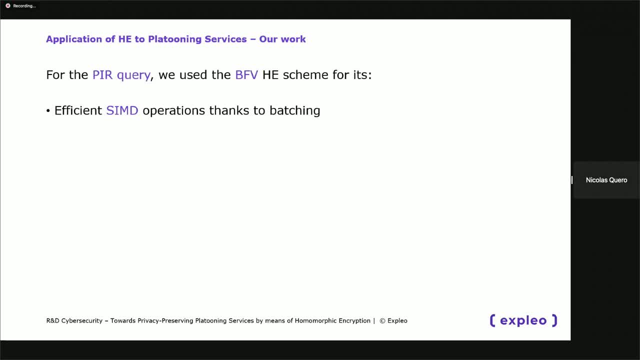 that. but we use pav because it allows for efficient simd operations thanks to patching and also it induces a natural key military user management without requiring to share any homomorphic public key on the server from any client. so that's pretty convenient. uh, the where what we do with the parameters we have? 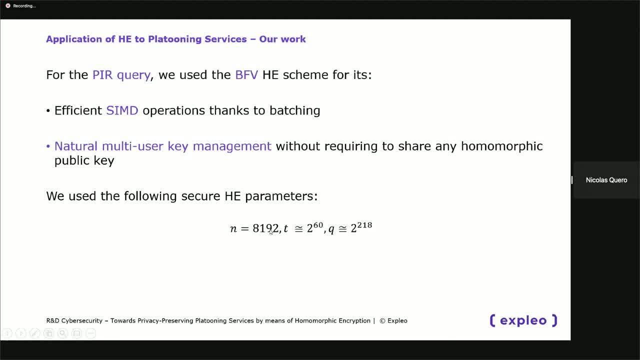 we could encode about 8 000 numbers of each 60 bits, and we we define in the paper how, how exactly we encode the, the sets of platforms, and how we many, and how we can open the other, the desired queries. another bfd, which is a homomorphic encryption scheme, can be replaced by: 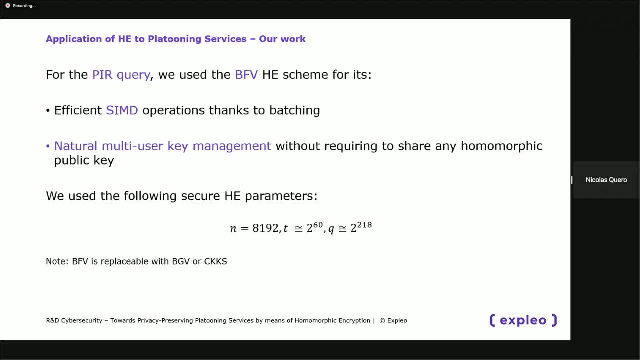 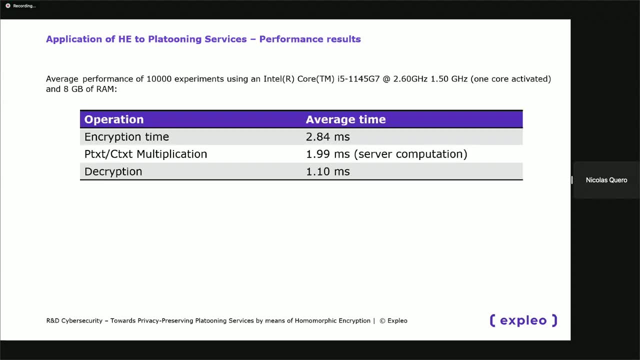 bjv or ckis or two, which are two other. how are morphic encryption schemes which allow them also for batching. so, in terms of performance, the most important point is the, the Bridge to all the ways to get the data out of the system versus the data and, but this is not always true. by the way, we have gonna examine this again and make a lot of changes in our 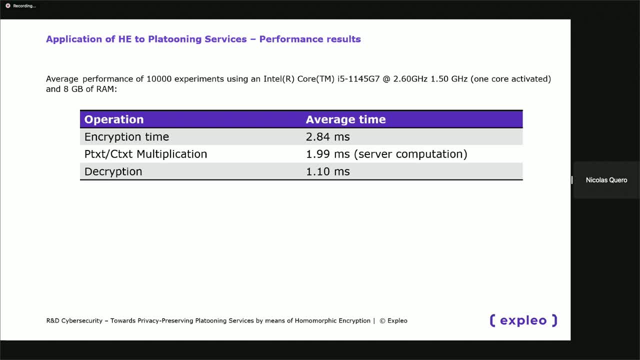 but this is not always true. by the way, we have gonna examine this again and make a lot of changes in our interesting number is the two milliseconds of server computation. uh, we, which should allow for about 500 queries per second on the on a single core, which can obviously increase a lot with. 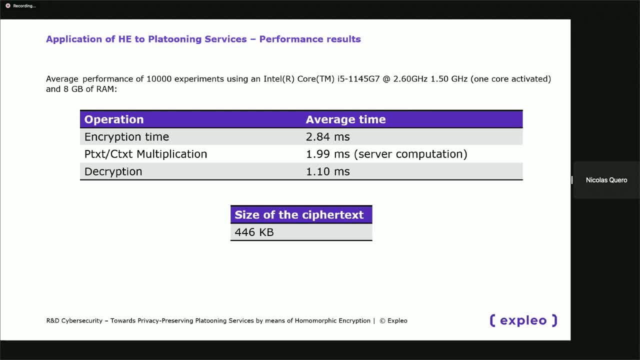 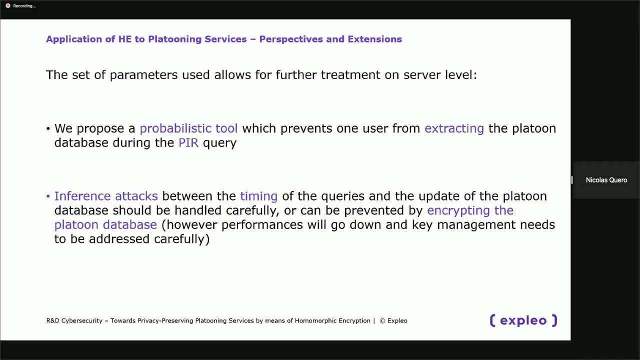 better resources and at the size of the ciphertext it can be pretty high. there is around 450 kilobytes go and return, so that's probably the the biggest cost in our protocol. i will also propose a probabilistic tool to prevent a user from extracting the database. 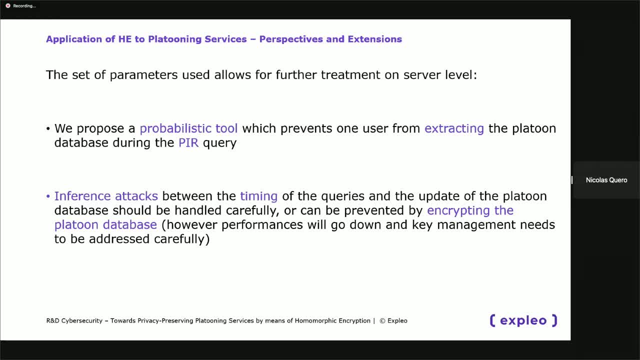 during a prior query, because during a pir query, because the data is encrypted, does the server cannot know whether the the data was set to or everywhere, except for one precise location. so we propose a probabilistic tool to prevent the user from setting once everywhere and thus extracting the database during the pir query. 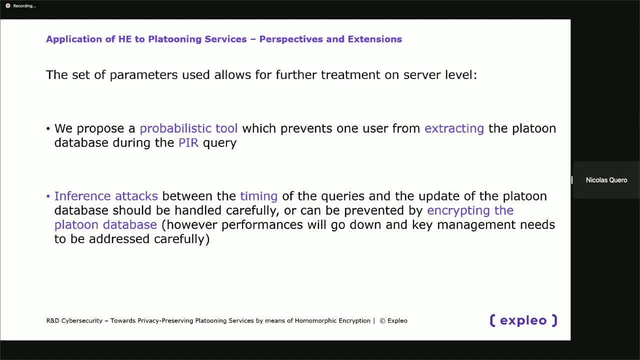 also some inference attacks can still be possible because the the query is encrypted but the database with the plateau is not, and then if a user performs a query, let's say at midnight, maybe 10 minutes after, the platinum database will be updated for one precise return and then the server could know that the user who made the query- uh, thanks for this precise. 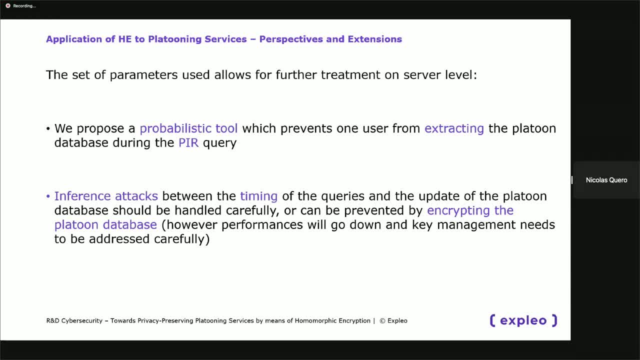 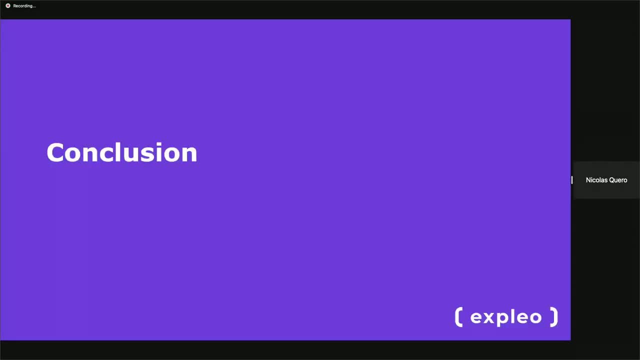 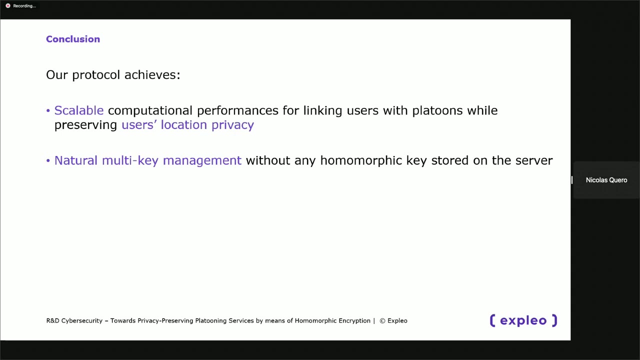 button or joined it. so this kind of attacks will need to be shuffled carefully and it can be prevented by encrypting the platinum database, uh. however, the performances will go down. then the key management will disappear. so we believe we we achieved a scalable computational performances to link users with platoons while preserving users location privacy.